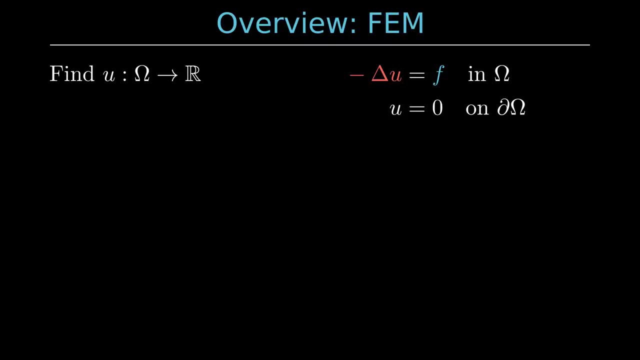 problem. description of the Poisson problem in what is called the strong form. In the second step, we then apply integration by parts to the strong form and arrive at an integral form of our PDE, the weak or variation form. In the next step, we make our function spaces finite dimensional to be able to work with. 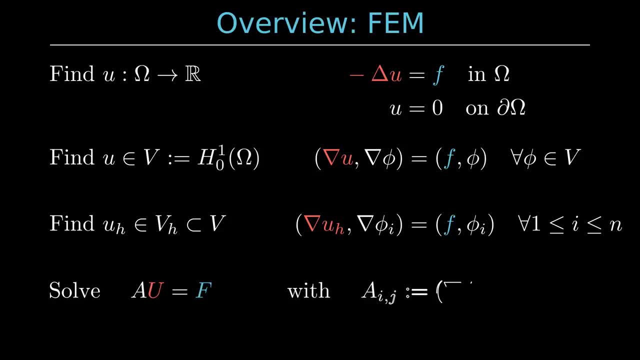 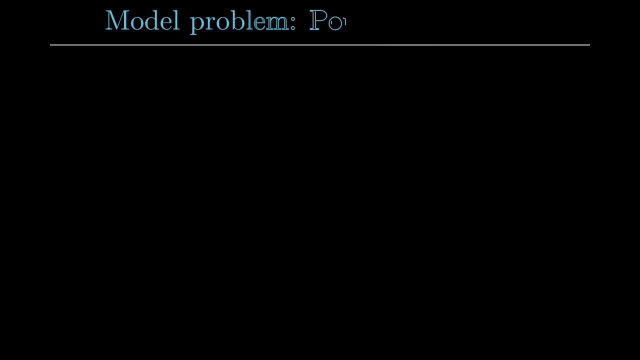 them on a computer. In the last step we then transform the discrete problem into a linear equation system. By solving this linear system we then get an approximate solution of our differential equation. Let's look at the familiar problem of Poisson's equation. 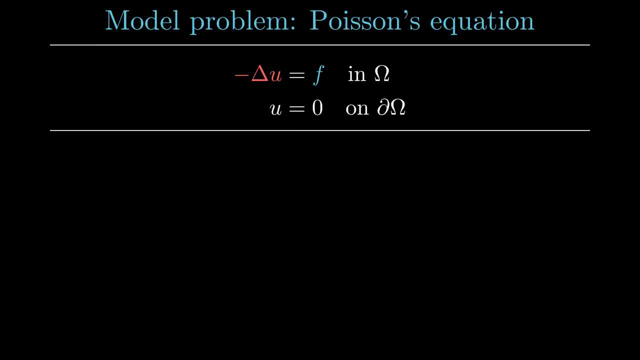 Minus Laplace. u equals f in the domain omega and u equals 0 on the boundary of the domain. Now we have to specify how the Laplace operator is defined. It all depends on the dimension d of the domain of the function, u. In general, the Laplacian of u is just the sum of the. 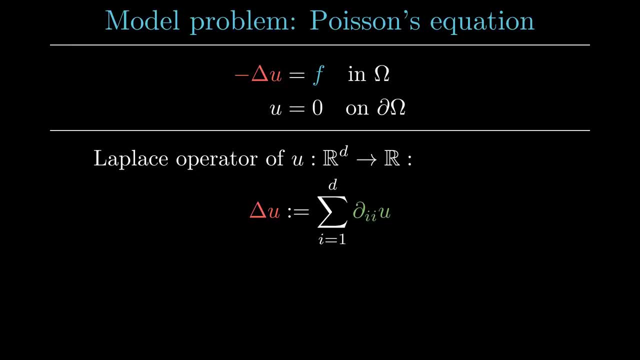 second spatial derivatives of u, Or more concretely: in 1D, the Laplacian is the second derivative. In 2D, the Laplacian is the sum of the second derivative with respect to x and the second derivative with respect. 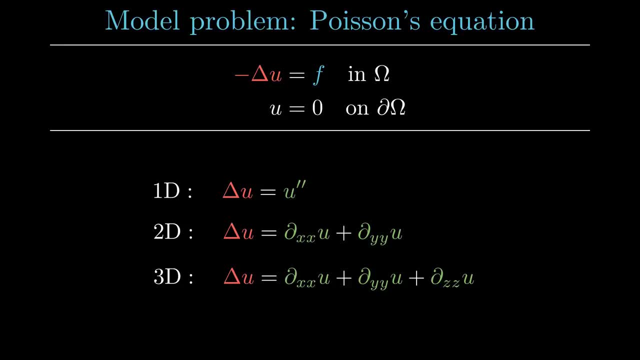 to y. In 3D, the Laplacian contains also the second derivative with respect to z. For the sake of simplicity, we will restrict our analysis to the derivative with respect to z. Therefore we can insert the definition of the Laplace operator into Poisson's problem. 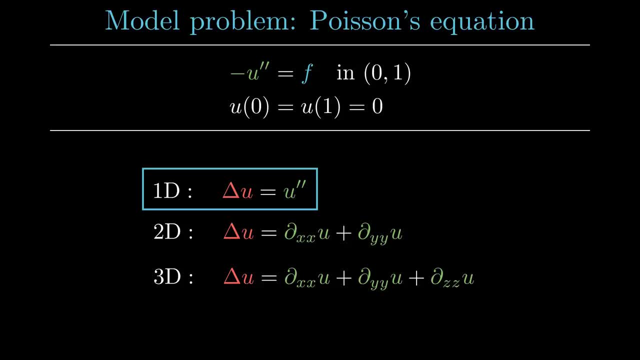 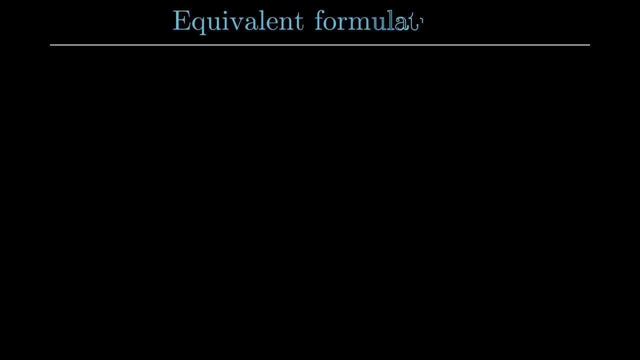 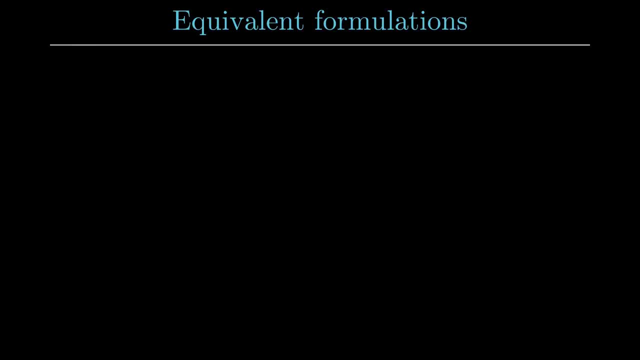 Let us look at some different forms in which it can be represented. But first we need to define some frequently used elements. This is our notation for a scalar product. The scalar product of two functions, v and w, is the integral of the product of v and w. 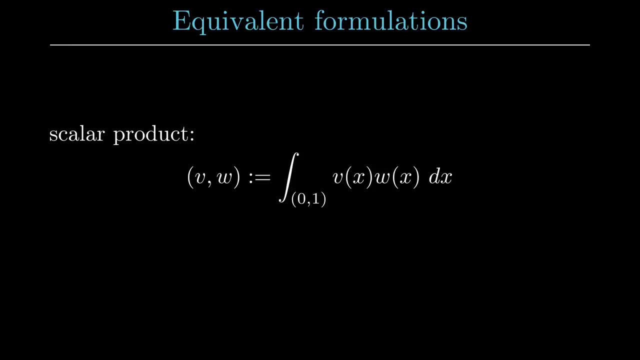 Here we integrate over the domain omega, which is the open interval from 0 to 1, making the Poisson equation. Let's look at some different forms in which it can be represented. The scalar product of two functions, v and w, is the integral of the product of v and w. 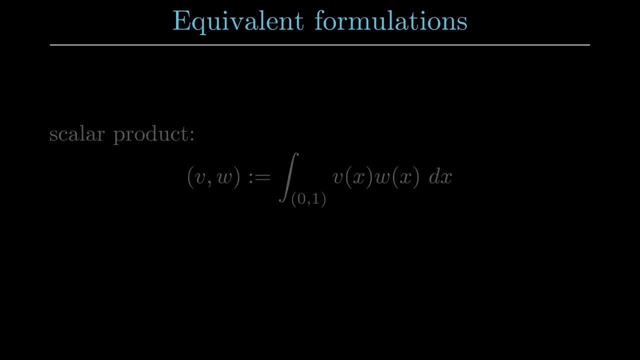 Additionally, let v be a function space which we will work with. This space contains all functions that are continuous and have a piecewise continuous and bounded derivative on the closed interval from 0 to 1.. Furthermore, these functions need to satisfy the boundary conditions that the function 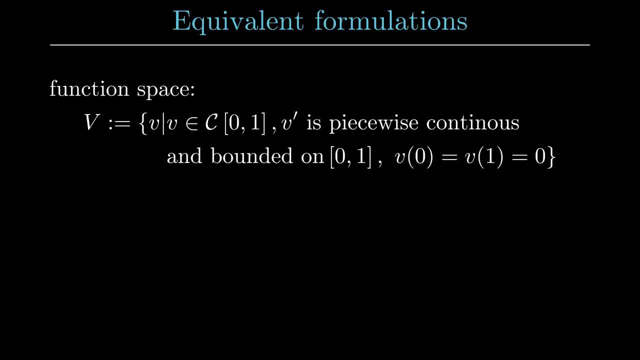 is 0 at the boundary of the domain. The energy functional is a mapping from our function space v to the real numbers. The formula for f of v is given below. Now we have all the tools needed to express the different formulations. We start with a strong formulation of the Poisson problem. 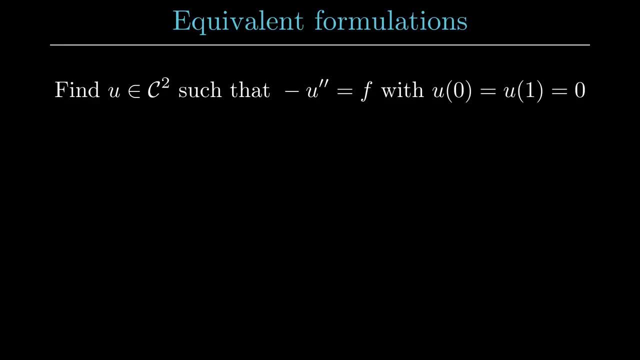 Here we are looking for a twice differentiable function. We start with a function u which satisfies the equation minus u, double prime equals f inside the domain and fulfills the boundary conditions u of 0 equals u of 1 equals 0.. The next formulation is the weak or variational form. 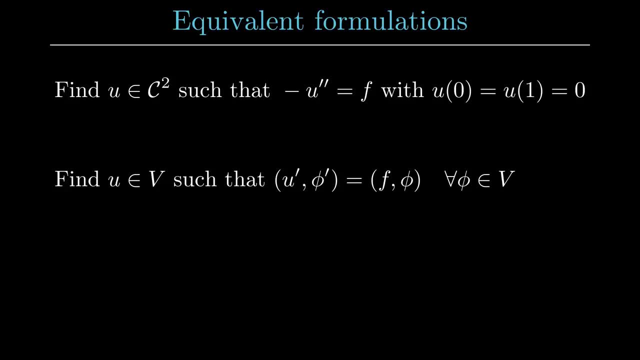 In contrast to the previous formulation, our solution u should now be the weak or variational form. In contrast to the previous formulation, our solution u should now be the weak or variational form. It should now be from our function space v and needs to fulfill the integral equation. 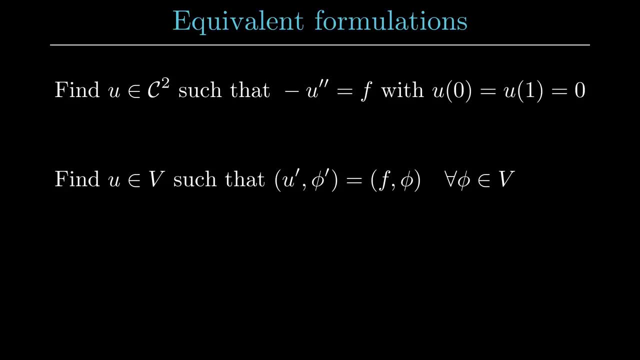 scalar product of u, prime and phi. prime equals scalar product of f and phi for all test functions phi from our function space v. The last problem statement is the energy minimization formulation. u and v should have the smallest value in the energy functional from all functions phi. 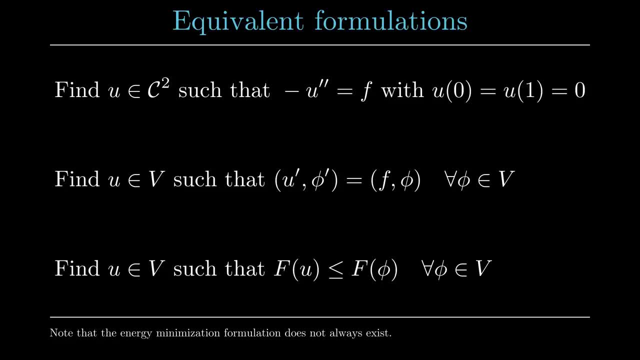 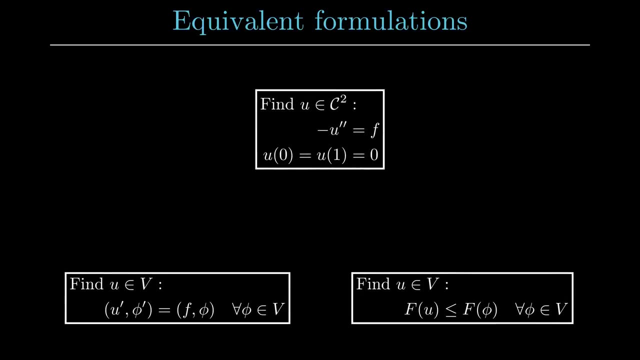 from the function space v. Please note that although this energy minimization formulation exists for the Poisson problem, it doesn't always exist for other PDEs. Let us now take a closer look at the first two formulations of the Poisson problem. 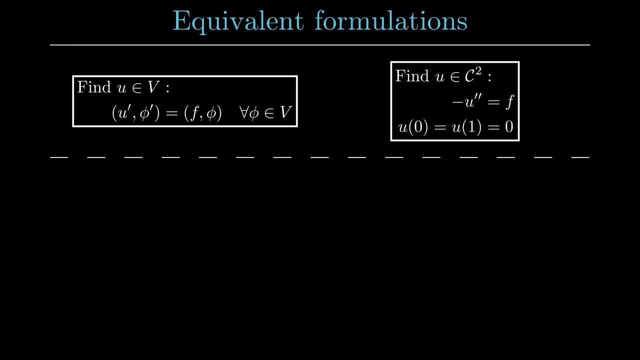 The first formulations are, of course, the weak or variational form. The second formulation is the weak form. The third one includes only the weak form. The fourth one includes only the weak form. The fifth one includes only the weak form. Let us start with the strong form and derive from it the weak form. 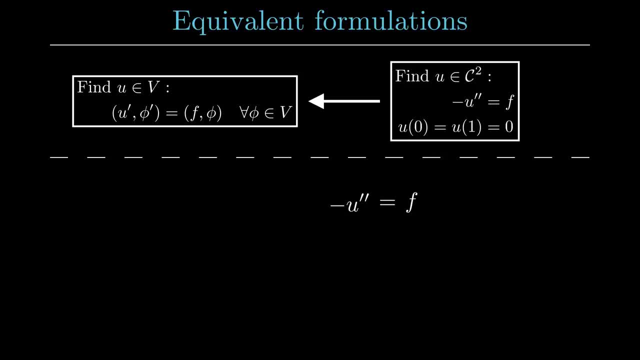 Let u be a solution of minus u. double prime equals f, The. this equation should still hold when we multiply from the right with a test function phi from v and integrate over the domain. The equation is therefore the least valid when we take the test function phi from v. 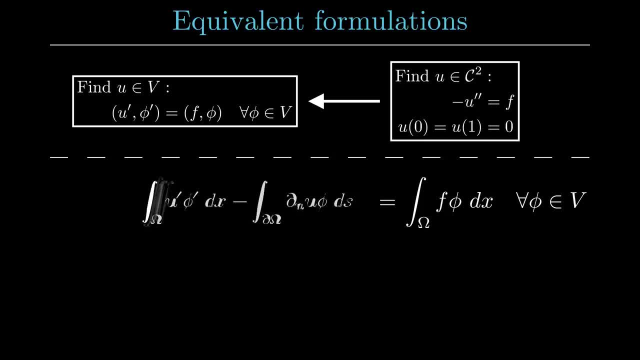 and integrate over the domain. We can now apply our test function phi from v to the stopping equation. Thank you very much for your attention. integration by parts to the left-hand side of the equation. Now we have almost arrived at the weak formulation. The only term that is bothering us is the. 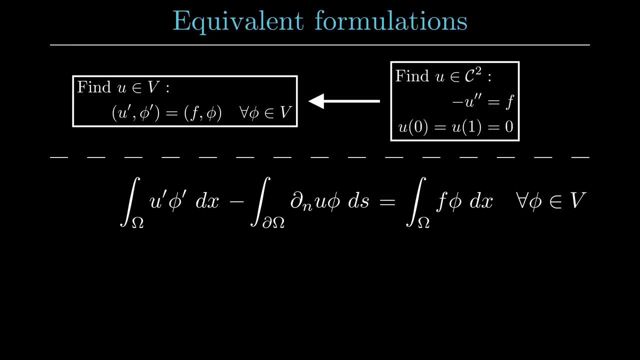 integral over the boundary of the domain. We can rewrite this integral by realizing that the boundary of the domain consists only of the point 0 and 1.. Luckily, we can go back to the definition of the function space V and use the fact that phi needs to satisfy the boundary conditions. Thus the 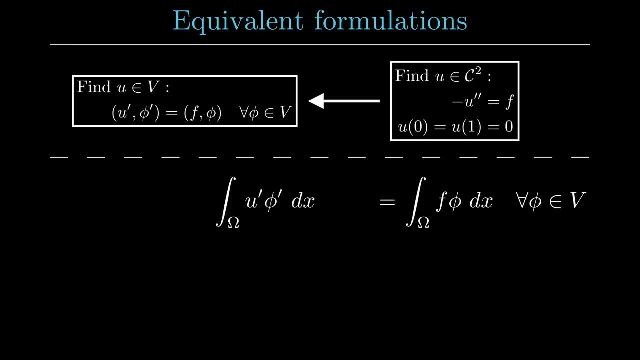 additional terms disappear due to phi of 0 equals phi of 1 equals 0.. Finally, we have derived the weak formulation. Now let us do the reverse and derive the strong form from the weak formulation. Let the integral equation scalar product of u prime and phi prime equals. 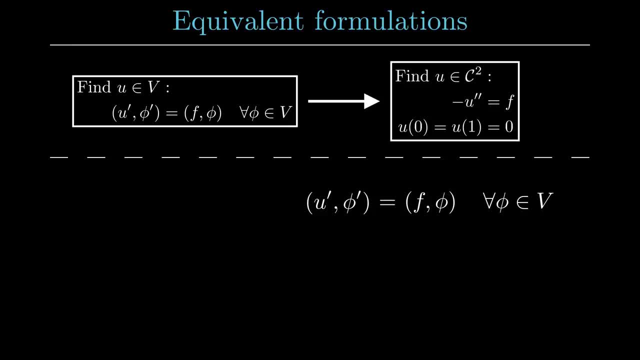 scalar product of f and phi be fulfilled by u. First we insert an artificial 0. We then again use that. phi vanishes at the points 0 and 1. This allows us to apply integration by parts. This time it is only the artificial. 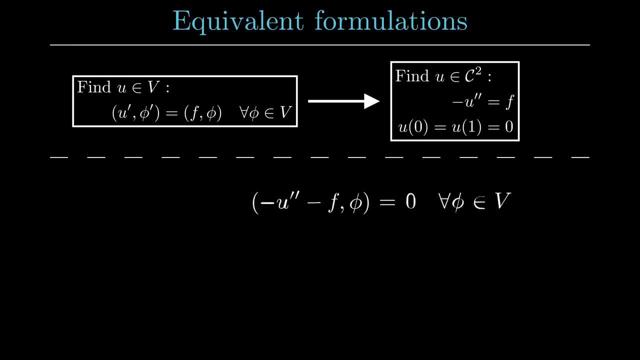 0.. We then again use that phi vanishes at the points 0 and 1.. This allows us to apply integration by parts. This time it is only the artificial 0.. We then again use that phi vanishes at the points 0 and 1.. This allows us to apply integration by parts. This: 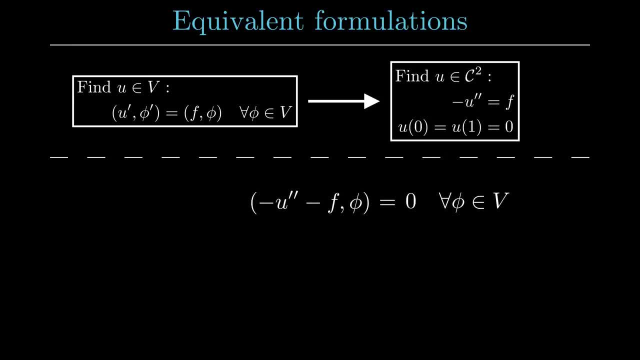 allows us to apply integration by parts. This allows us to apply integration by parts By bringing the f to the left-hand side of the equation. it holds that the scalar product of minus u, double prime, minus f and all test functions phi equals 0.. 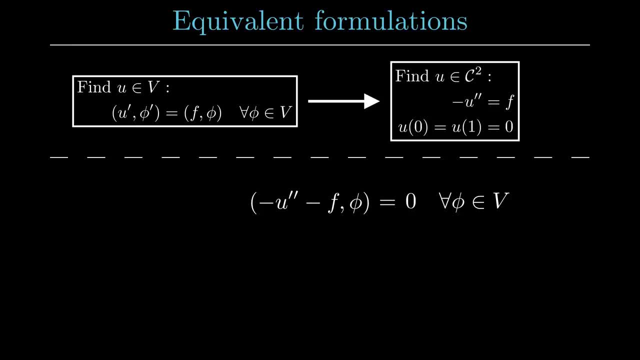 This can give us the strong formulation when we reach into our mathematical toolbox and get a hold of the fundamental lemma of calculus of variations. This lemma tells us that if a continuous function w equals 0 when multiplied with some test function phi and integrated over omega, then the function w itself must. 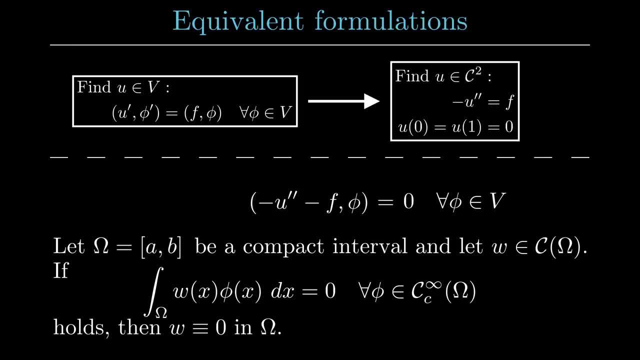 be 0.. In this lemma, the test function space is the space of all infinitely differentiable functions with compact support. This means that these functions vanish after some time and are void after some time, and are void after some time and are void after become zero. Having applied the fundamental lemma of calculus of 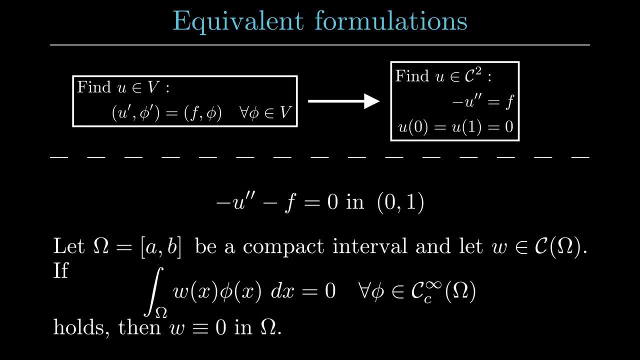 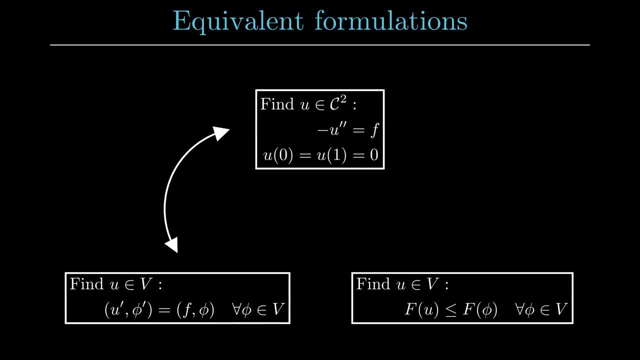 variations, we recover the strong formulation. We have thus shown that the strong and the weak formulations are truly equivalent. Additionally, it can be shown in a straightforward manner that the weak formulation and the energy minimization formulation are also equivalent. Overall, this means that all 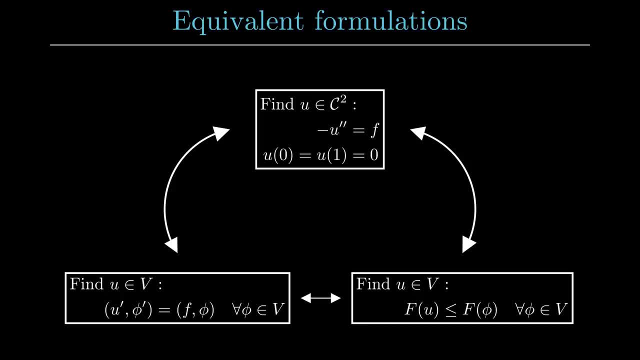 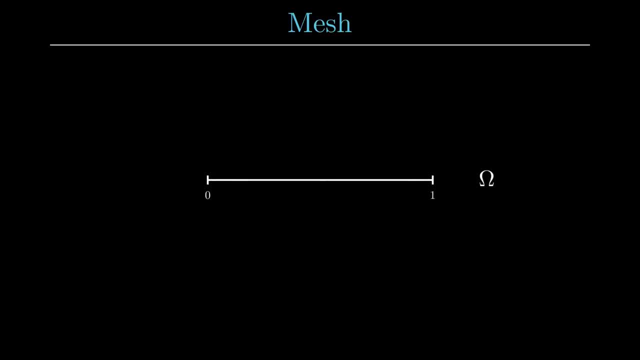 three formulations of the Poisson problem are equivalent. To achieve a computable solution, we will need to spatially discretize the physical domain- in our case the interval from 0 to 1, into a mesh of only a finite amount of nodal points xi. 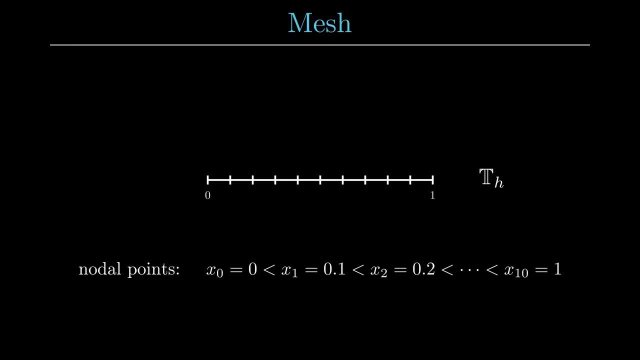 We choose the mesh parameter, h being equal to 0.1.. If we now look at a cell of the mesh, in our case an interval from xi to xi plus 1, we can define what a finite element is. The finite element is a triple k pk sigma, where k is an. 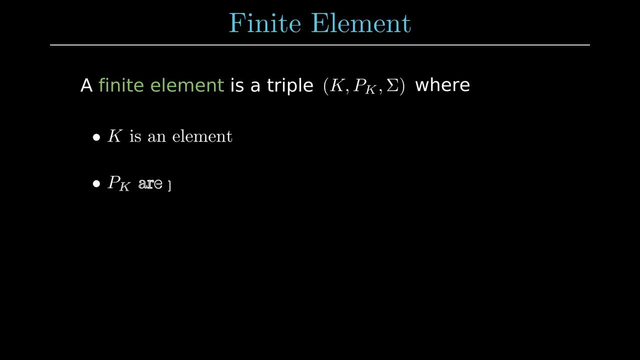 element or a cell of the mesh. pk are polynomials on this element: k, and sigma is a set of degrees of freedom, or short dooF. We saw what an element of the mesh is, but what are those polynomials and degrees of? 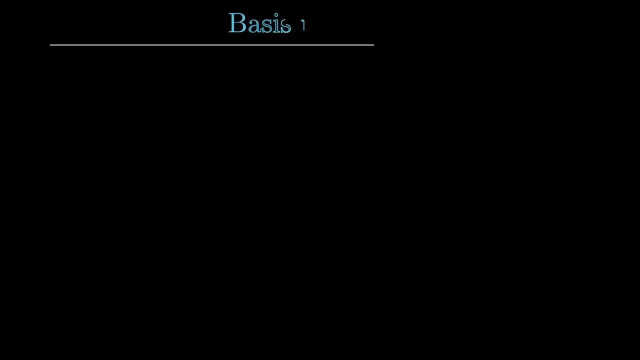 freedom. and why do we need them? In order to reduce dimension of the infinite dimensional function space V, we can define a finite dimensional subspace Vh, which consists only of functions that are polynomial on each element k of the mesh and still fulfill. 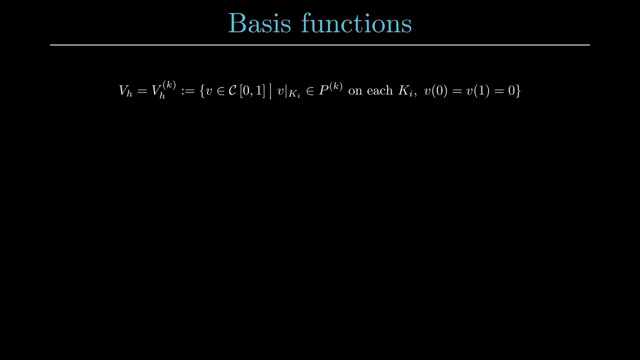 the property of being zero on the boundary. Since this space is finite-dimensional, we can look at a function vh and construct its unique basis representation with the basis functions phi0 to phi10,. a property that the ith basis function should yield is that on the ith degree of freedom, it should be 1 and 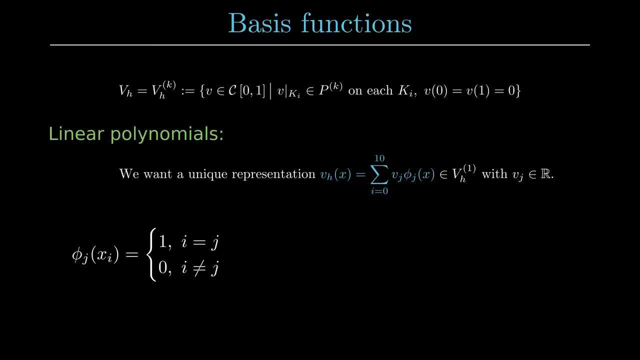 on all other degrees of freedom, it should be 0.. In the case of linear basis functions, the degrees of freedom are simply the nodal points xi and xi plus 1 of the mesh. But in the case of higher-order polynomials, the degrees of freedom are the support points. 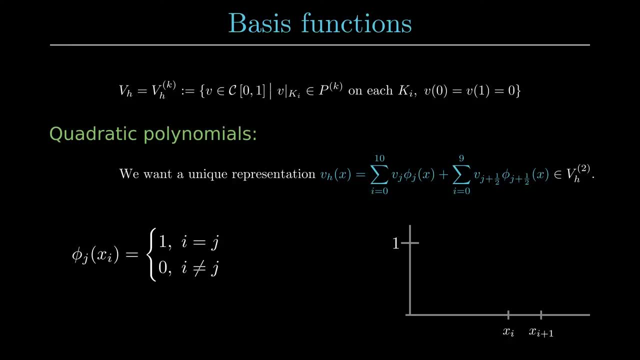 needed to achieve this, To construct a polynomial of the required order. For example, in the case of quadratic basis functions, we need to add a third degree of freedom- xi plus 1 half- to construct those There. we also have additional basis functions- phij plus 1 half. 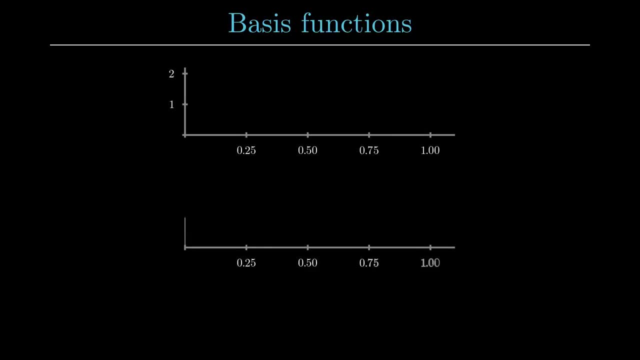 Let us now take a peek at how we can decompose functions vh and phi0.. First, we need to add a third degree of freedom xi plus 1 half to construct the linear basis functions. For this we need to add a third degree of freedom xi plus 1 half to construct those. 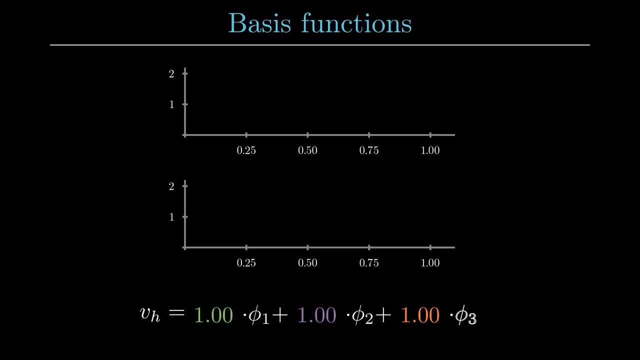 For this, let vh be simply the sum of our three basis functions. In the upper graph, you can see the function vh. In the lower graph, you can see the basis functions with their respective scaling. We start adding the linear basis functions Which, due to their shape, 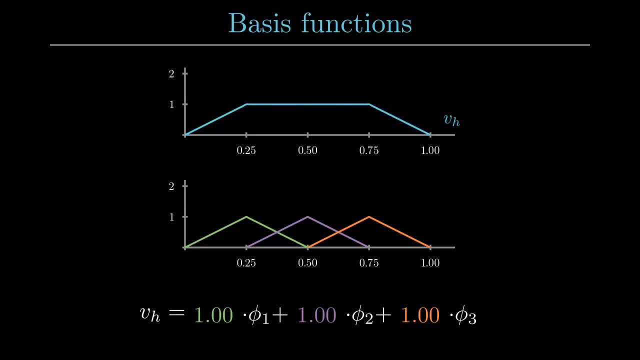 their shape are also referred to as head functions. We see that VH vanishes at the boundary and has the same value as the corresponding basis function at the nodal points. In between nodal points, the values of VH are a linear interpolation between the values. 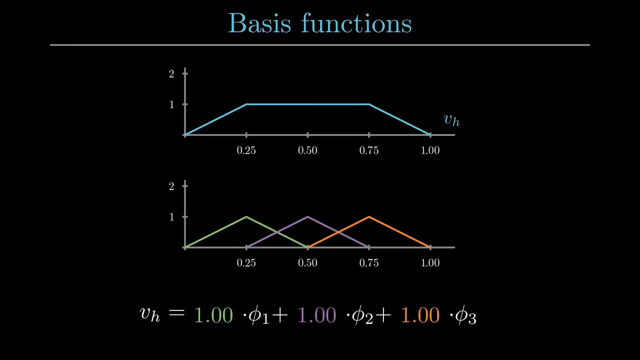 at the nodal points. This fact and the contributions of the individual basis functions can better be seen when we vary the coefficients in front of the basis functions. We have thus shown that all functions in VH can be constructed when we just play around. 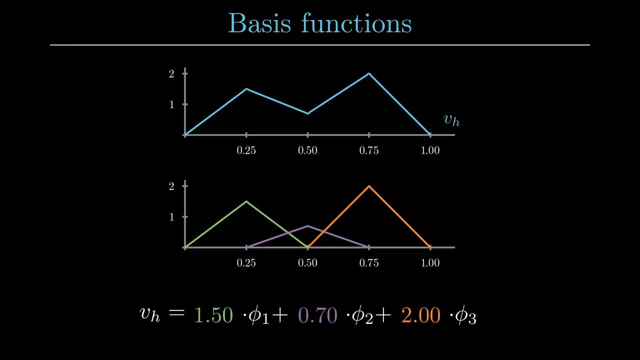 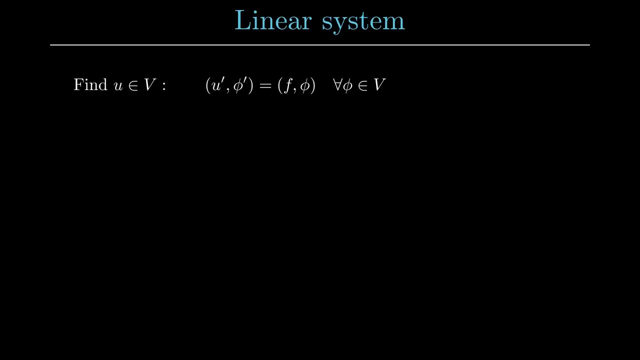 with the coefficients. in front of these basis functions, A question that you might be asking yourself right now is: What is the value of VH? What are these basis functions good for? Well, instead of solving the weak form which we have been talking about previously, we 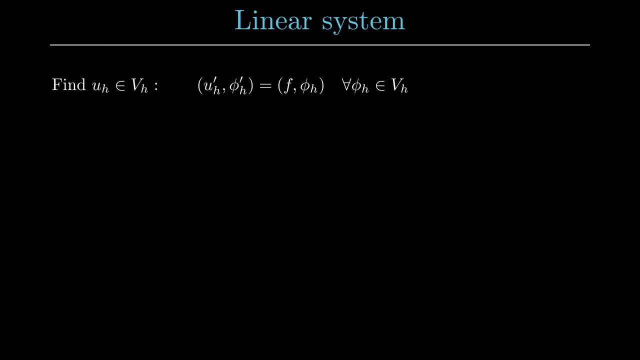 now work with a discrete function: space VH instead of the infinite dimensional space V. This is much easier to do with a computer, since there are only finitely many basis functions- phi, j- And we now just need to find the basis functions. We find the real numbers, uj. 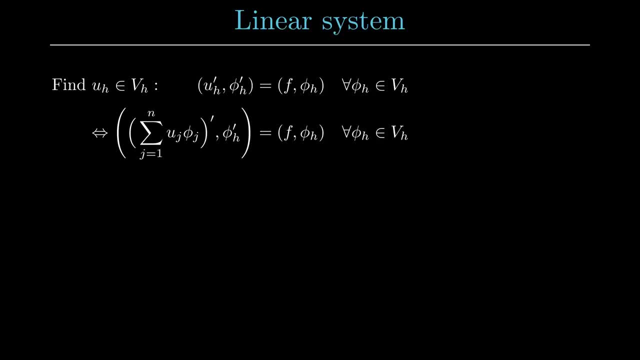 We insert this decomposition of uh into our discrete weak form, Then we can take the summation out of the scalar product due to the linearity of the derivative. In the next step, we can also decompose phi h into its basis functions, phi i. 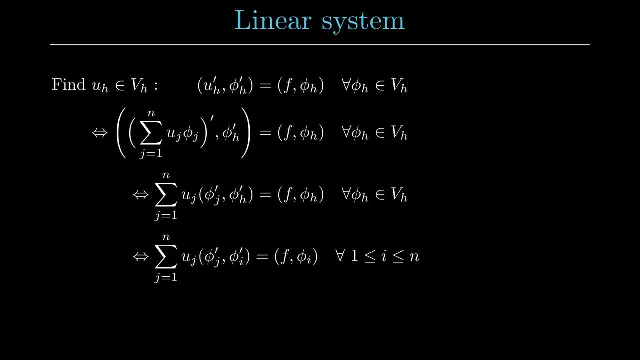 If the equation holds for all basis functions phi i, then we can also decompose phi h into its basis functions phi i. If the equation holds for all basis functions phi i, then we can also decompose phi h into its basis functions phi i. 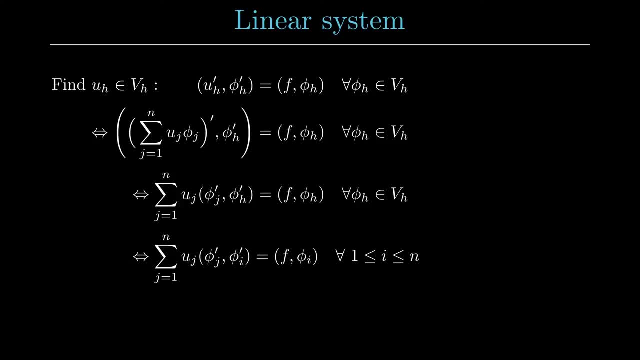 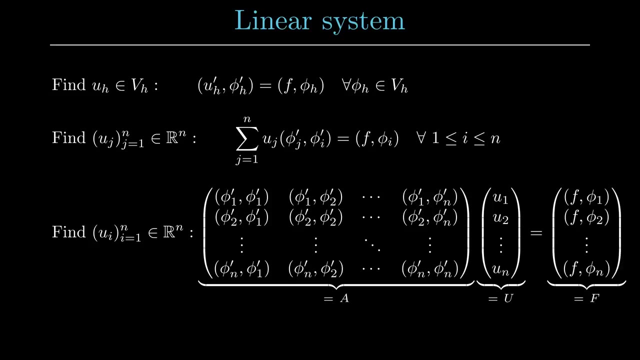 Then, due to the linearity of these equations, it must also hold for our test function phi h. This problem statement can also be written in matrix notation and is shown in such a form below: Note that when we constructed the matrix, we used the property that the matrix is symmetric. 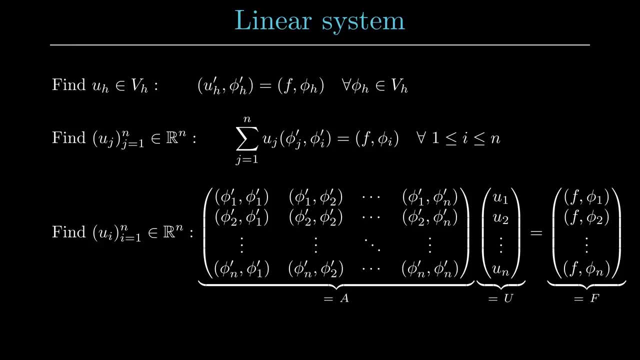 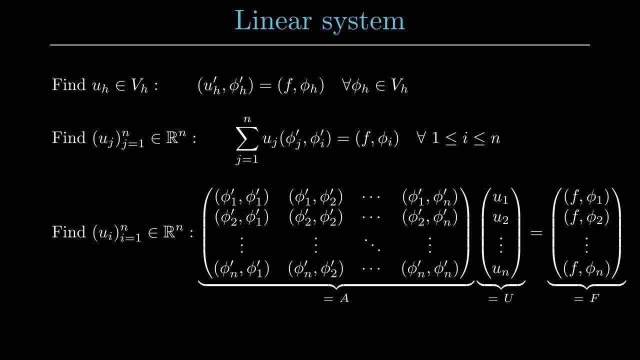 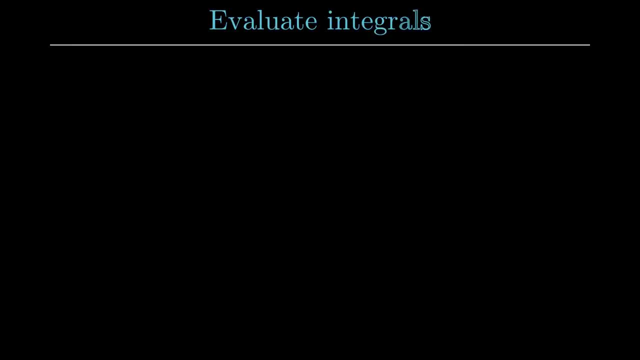 the strong form of the Poisson problem. Now we only need to solve this linear system for the solution vector u. However, in the matrix formulation there are still a lot of integrals that we need to evaluate first. Now we will dive into how those integrals can be evaluated when working with linear. 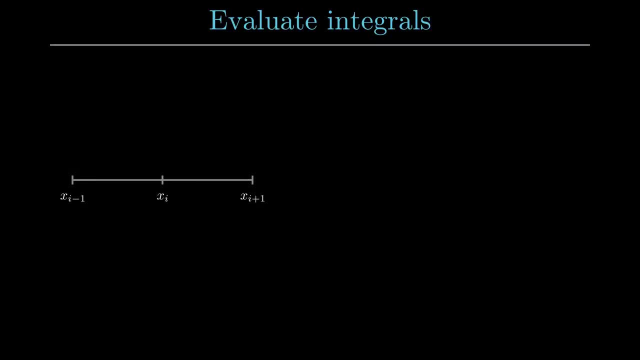 finite elements. For this purpose, let us look at three consecutive basis functions. The dashed lines represent their derivatives, which are piecewise constant, and take the values 0 and plus or minus 1 over h. Now we will compute a 3 by 3 sub-matrix of A in which these basis functions come up. 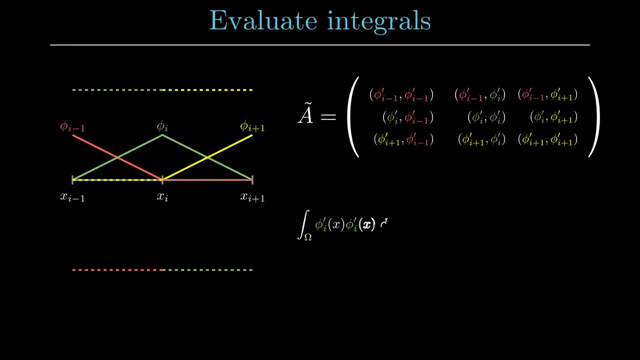 Let us first calculate the diagonal entries by looking at the entry in the matrix as a pair. Any derivative of the middle of the matrix, The ith basis function, is 0 outside of the interval from x to x. Thus we only integrate over this interval. 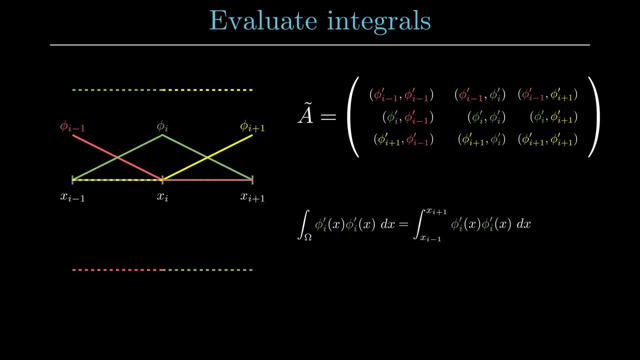 This interval is then divided into the two cells on which the derivative of the basis function is constant, namely plus or minus 1 over h. Further simplifications lead to the value 2 over h. Consequently, we now know the diagonal entries of our matrix A. 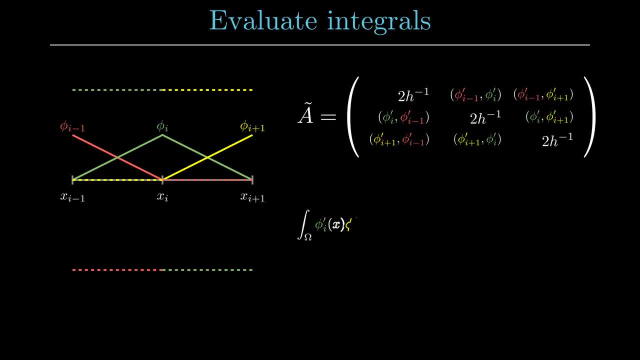 What are the values of the entries which are exactly one left or one right from the diagonal of our matrix? We again use that the ith basis function is zero outside of the interval from x to xi plus one, but the i plus oneth basis function is zero on the interval from xi minus one. 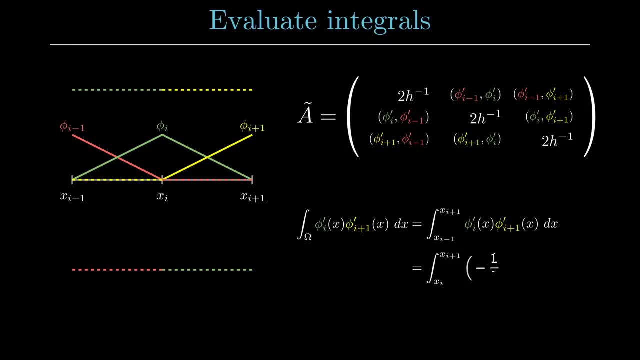 to xi as well. Thus we only integrate over the cell from the ith to the i plus oneth nodal point. Inserting the derivatives and evaluating the integral then gives us minus one over h for the entries right next to the diagonal of A. 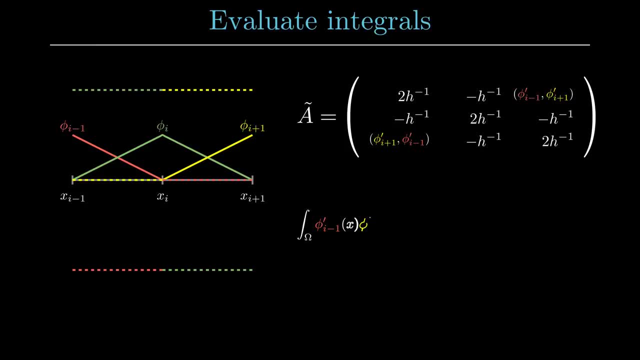 What about the entries? What about the entries of the matrix which are further away from the diagonal? In the example of the i minus oneth and the i plus oneth basis function, we see that these integrals all have to be zero because such basis functions don't share a common interval. 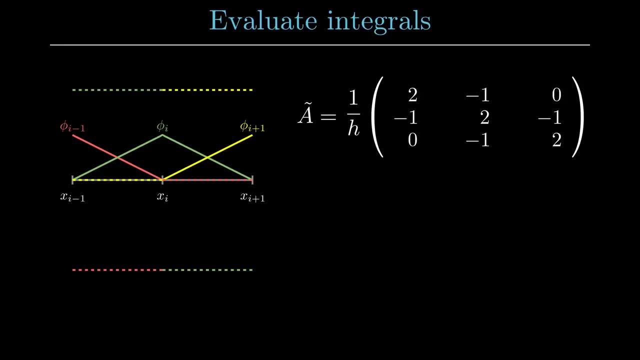 on which they are non-zero. The system matrix A is thus sparse, which means that it has only very few non-zero entries. Similarly, we can evaluate the integrals that make up the right-hand side. First, we need to know the function f from our Poisson problem. 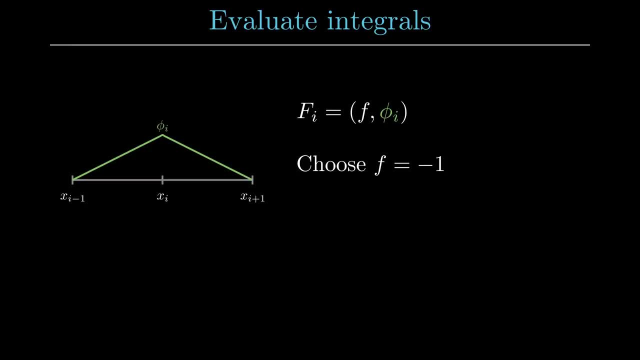 For the sake of simplicity, we choose: f equals minus one here. Through a simple integral, we see that the entries of f all evaluate to minus h. Finally, we can write down what the system matrix A is. Finally, we can write down what the system matrix A is. 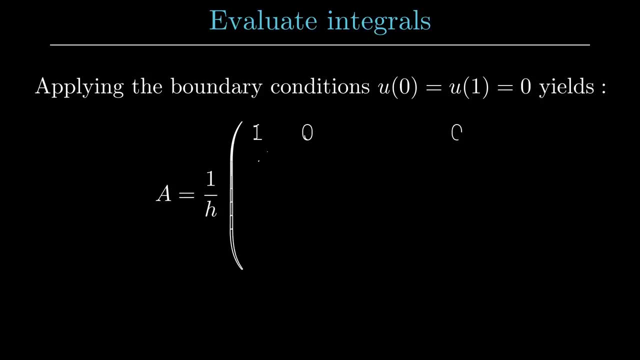 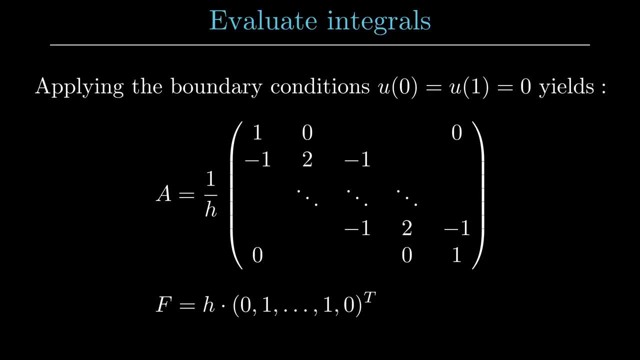 U a Q ay, Q ay U a Me a 터. absoluto Q u, Q u Ab drauf, Q u Tab fors Showerbill, Showerbill, Showerbill, Or again Ma-Riv, уб вещ beh. 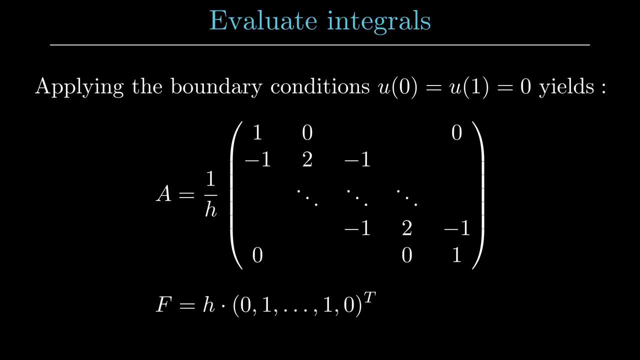 K, v woh, Su, b biv, K, pp, X, kp, X1, qt, K, kt, Muv, X, tu, tnl, X, WQ, which correspond to the nodal points at 0 and 1, we enforce on the matrix A and the vector F. 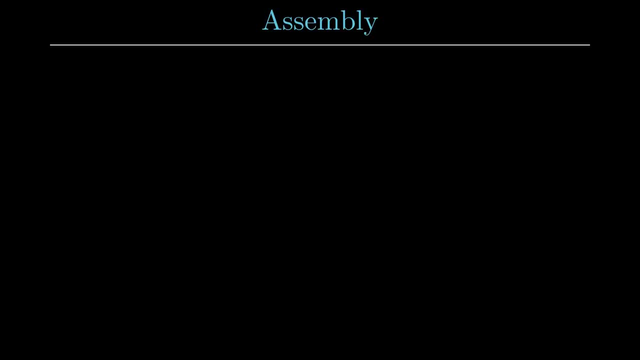 that the boundary conditions should be satisfied, Aren't we done now? We transformed the Poisson problem into a linear system and can now compute its solution, But we computed the linear system by hand, which can become very cumbersome for more complex PDEs. Therefore, let us create a step-by-step guide. 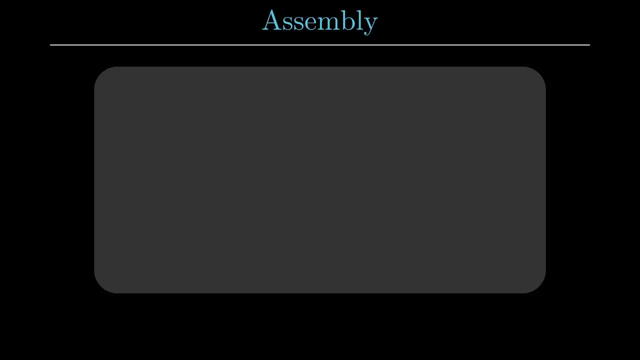 with which we can teach the computer to assemble the linear equation system for us. The simplest algorithm to do so is as follows. First, let us iterate over all elements k in our mesh. From now on, all our integrals won't be in the same order. 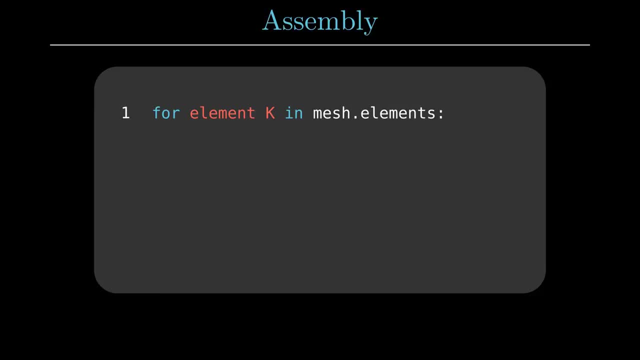 They won't be over the entire domain omega anymore, but only over one such an element k. The last thing needed for the evaluation of the integrals are two iterators over the degrees of freedom on the element k For our dofs i and j. 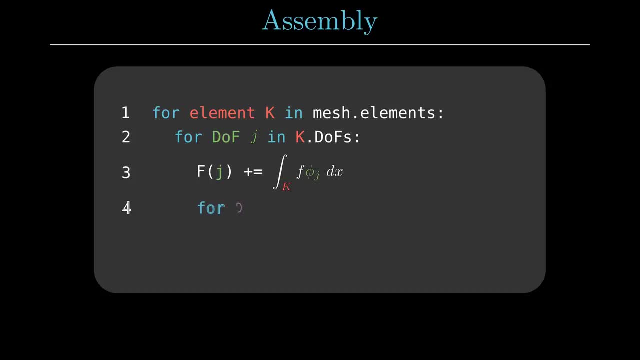 the corresponding basis functions phi j and phi i should be non-zero on the element k. With that we can compute f and a At this point. you might still be unhappy with our algorithm, though, since we haven't discussed how the computer should evaluate the integrals over a single element k. 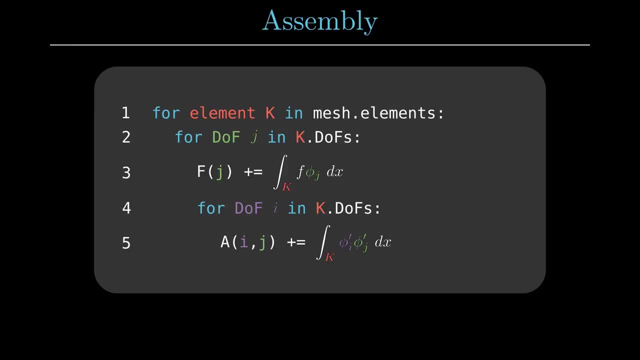 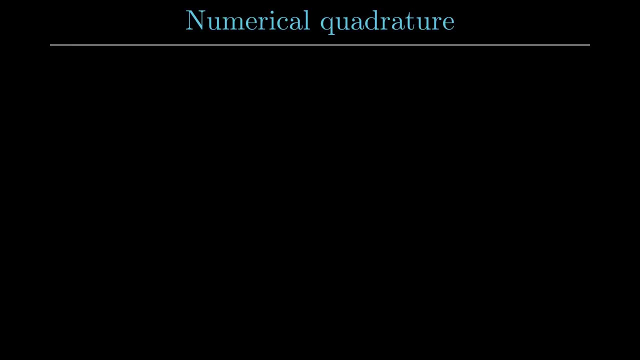 Should this be done analytically, the same way that we did it by hand? No, Luckily we can use numerical quadrature instead of computing all integrals exactly, which might often be very difficult. Let some function g be given, which should be integrated over some domain: omega. 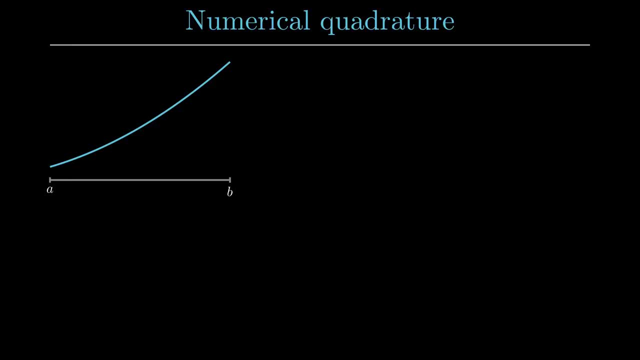 In our example, g is a parabola and omega is the interval from a to b. The general formula for numerical quadrature reads: The integral of g over the domain omega can be approximated by the sum of g over the domain alpha, evaluated at some quadrature points, Pl and weighted by some. 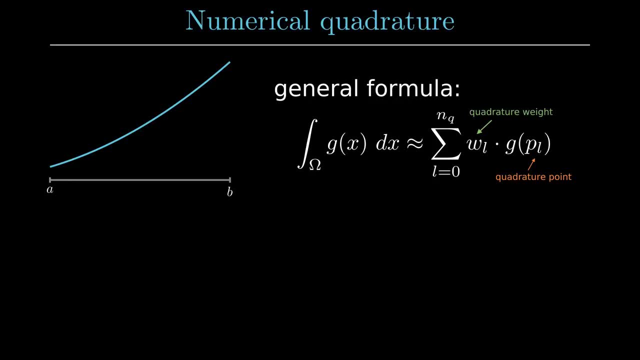 quadrature weights W. How this abstract formulation looks in practice is shown at the following examples. A simple method for numerical quadrature is the left-box rule, where the integral over the interval from a to b is approximated by the value of g multiplied by the width of the interval. 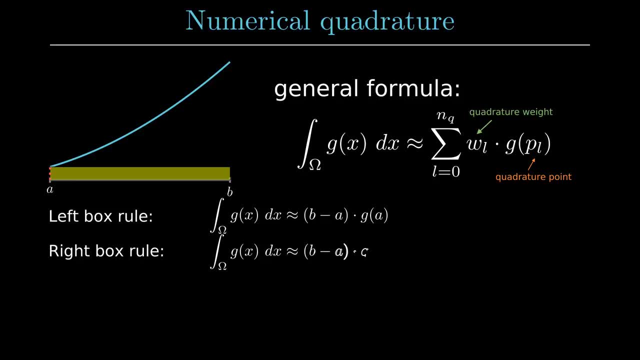 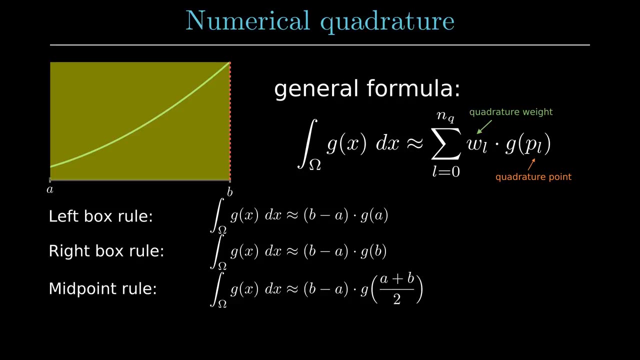 The right box rule works the same way, but we use the right boundary as our quadrature point instead of the left boundary, as in the case of the left box rule. The midpoint rule also only differs from the previous methods by a different choice of a quadrature point. 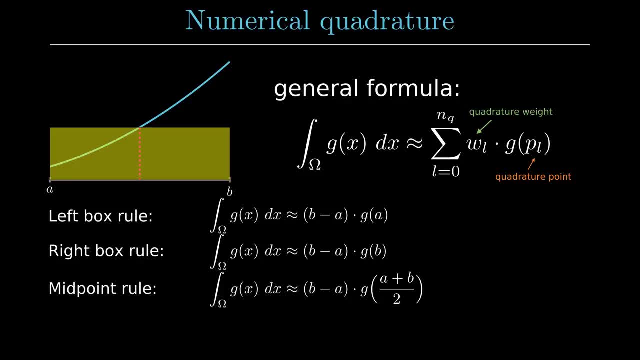 Here g is evaluated at the midpoint from the interval from a to b. In the trapezoidal rule we average over the values of g at the left and right boundary of the interval and multiply by the width of the interval, As you can see in the graph. 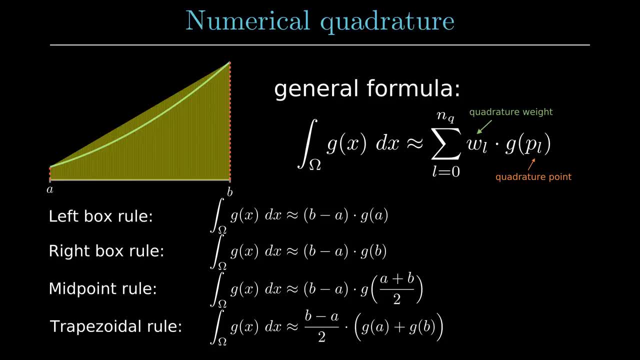 not even the trapezoidal rule computes the integral over g accurately. Therefore, in practice, we use higher order numerical quadrature with more quadrature points. There are different formulas depending on up to which degree of polynomial you would like to integrate exactly. For example, the trapezoidal rule can integrate constant and linear functions exactly. 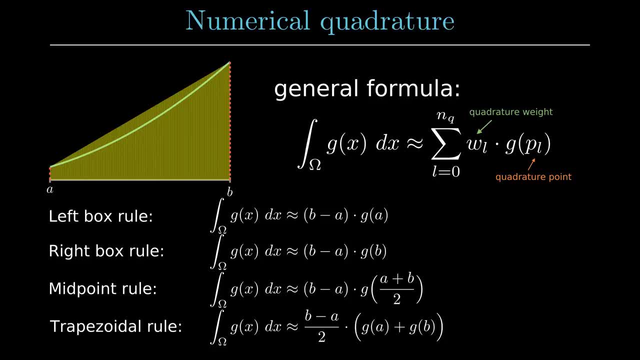 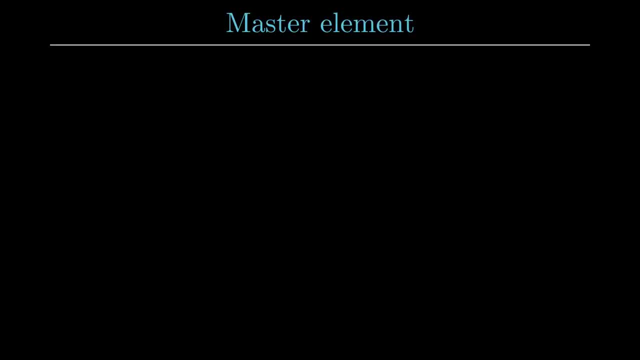 but is not accurate anymore when dealing with polynomials of degree 2 and higher. The last tool in our numerical integration toolbox is the transformation of the integral over individual elements into integrals over reference element, which is often called the master element in the literature. 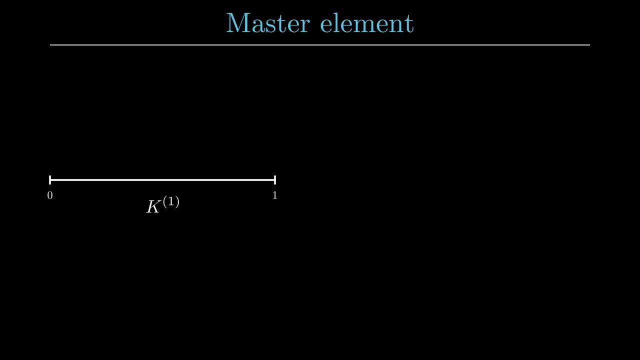 In 1D the master element is the open interval from 0 to 1.. First we define a linear transformation, th, from the master element k1 to a single element, ki. By j we denote t, which is the determinant of the Jacobian of this transformation. 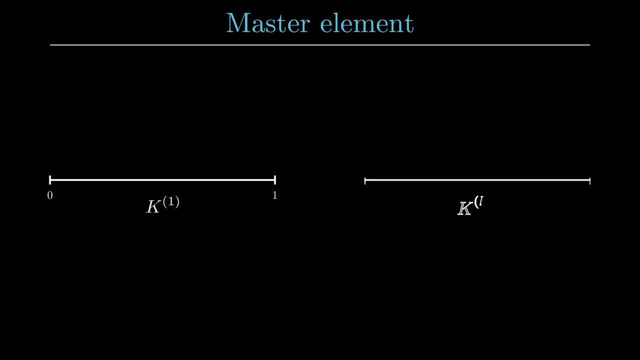 Similarly we also define the linear transformation back to the master element. the inverse of th, The derivative of this transformation, is given in the upper right corner. Additionally, to evaluate a given basis function on the ith element, we can first map back to the master element. 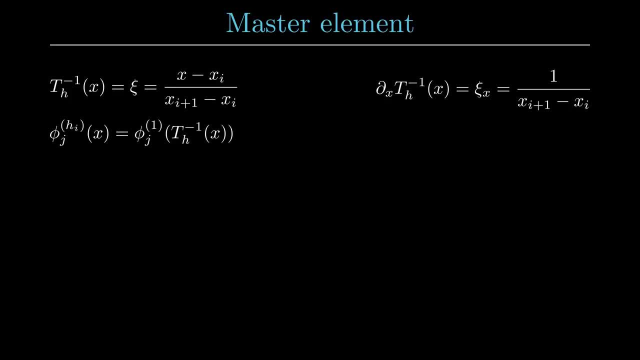 and evaluate the corresponding basis function, which is defined on the interval from 0 to 1.. Lastly, for further calculations we need to write down an expression for the derivative of the basis function on the ith element. Here we simply apply the chain rule to the previous equation. 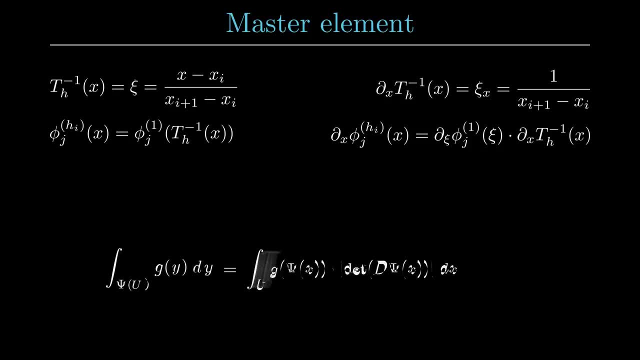 Starting with the change of variables formula, using our equations from above and numerical quadrature, we can thus make the integrals that arise in the matrix A and the vector F computable for a computer. Having done all this analysis of the Poisson problem, 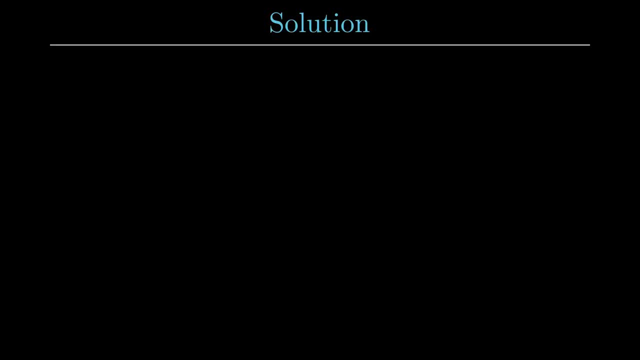 we now can solve it and visualize its solution. But first I would like to remind you that we chose F equals minus 1 in our problem formulation. This problem is sometimes also referred to as the closed line problem, Since we are modeling a closed line that connects the points and 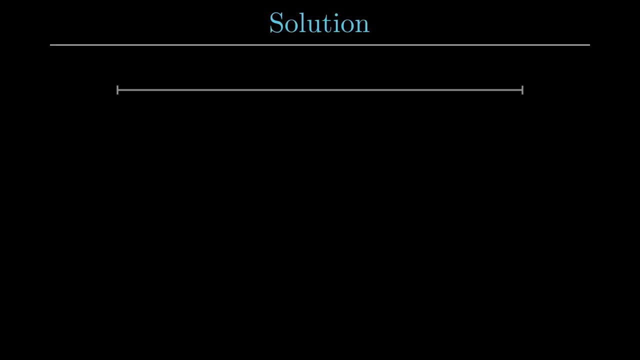 and we have gravity which is uniformly pushing the closed line downward. this is what our approximations of the physical phenomenon look like for various mesh sizes. As you can see, the approximations converge to the parabola 1 half times x times x minus 1,. 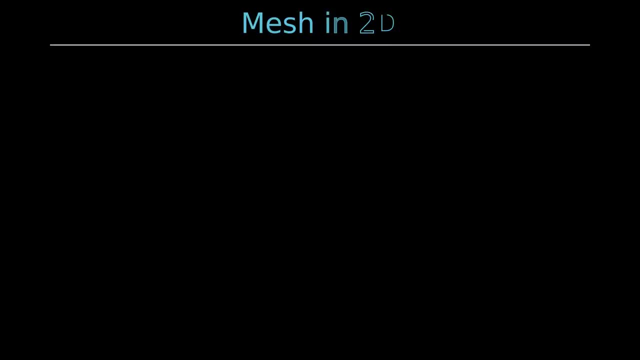 if we decrease the mesh size. The finite element method can also be used in 2,, 3 or more dimensions. We will briefly discuss the differences of the FEM in higher dimensions to the one-dimensional case. We will therefore deal with the Poisson problem in two dimensions. 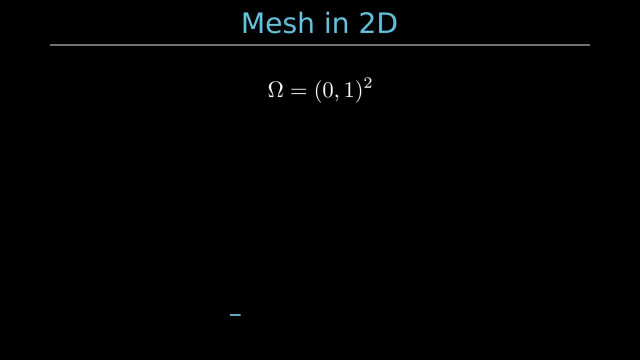 We choose the domain omega to be the unit square, Then we can decompose the domain with a given mesh size. for example, h equals one-eighth. The most interesting change between the finite element method in one and two dimensions is how the basis functions are being constructed. 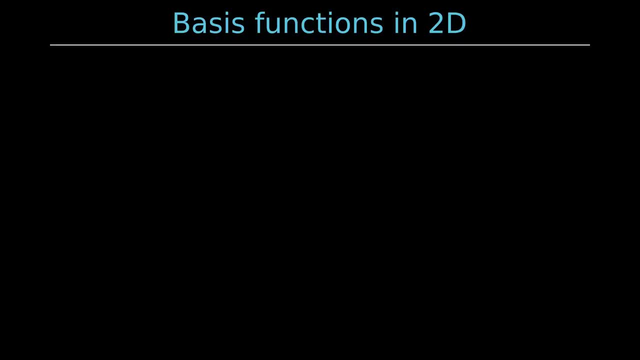 To construct linear finite elements in 2D, we could again look for functions that equal 1 in one corner of the unit square equals 0 at the other corners and are linear in x and linear in y. However, we now have a neat trick. 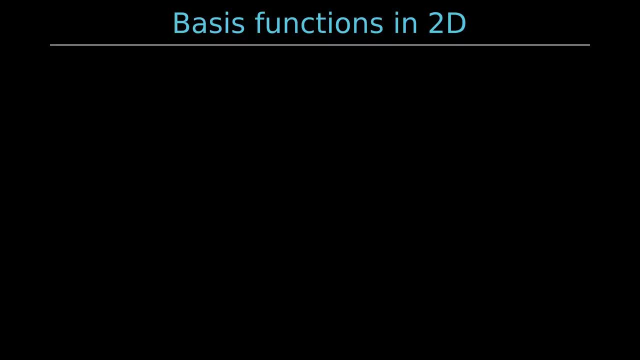 on how to construct our two-dimensional basis functions from their one-dimensional counterparts. We just need to compute the tensor product of the one-dimensional basis with itself to get the two-dimensional basis. This can be seen in the following visualizations: As usual, we assemble our linear system. 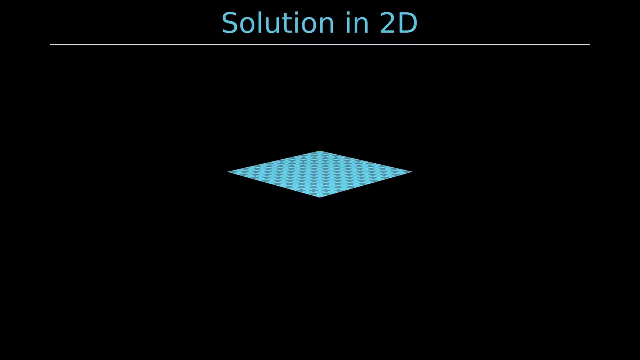 linear system and solve it Here. we used f equals minus one and are dealing with a similar problem as we had with a clothesline. in one dimension, Gravity pulls a square shaped piece of cloth downwards uniformly. This can be seen very well in our FEM solution. 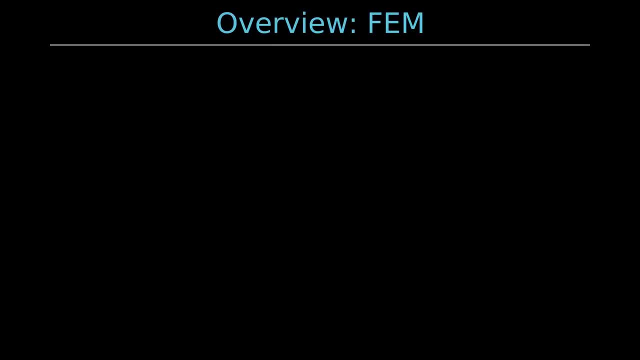 Finally, let us recap which steps we need to follow in the finite element method. First, we need to define the strong form of the PDE, which we are trying to solve. In this video we dealt with the Poisson problem. In the second step, we then apply integration by 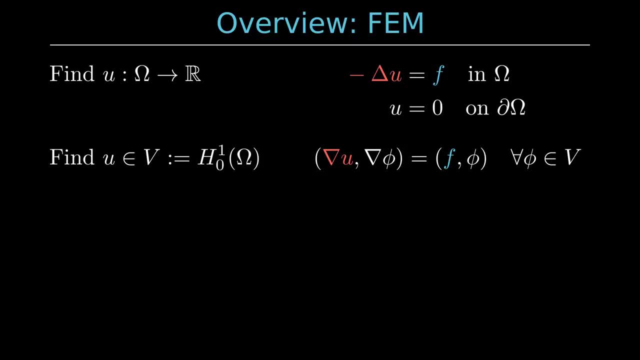 parts to the strong form and arrive at an integral form of our PDE, the weak form. In the next step, we make our function spaces finite dimensional to be able to work with them on a computer. In the last step, we then transform the discrete problem into a linear 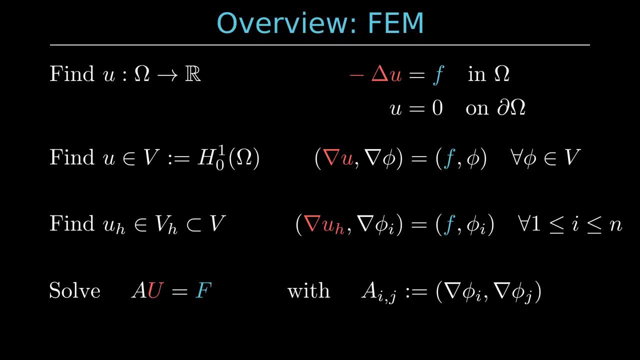 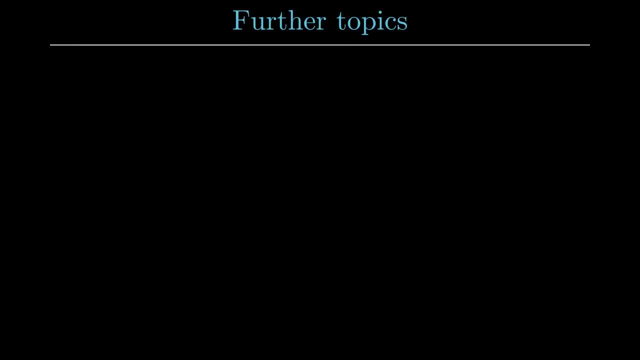 equation system. By solving this linear system, we then get an approximate solution of our differential equation. There are many further topics which might be of interest for you if you want to learn more about the finite element method and how it can be used. Firstly, you might want to look into more efficient ways of solving linear systems. 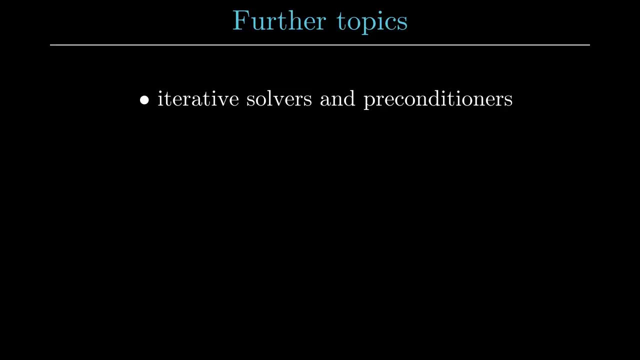 In high school, students learn about Gaussian elimination to solve linear systems. This corresponds to solving the linear system via LU factorization. Direct methods like this are not feasible if the linear system becomes very large. Thus it is useful to learn about iterative linearization. 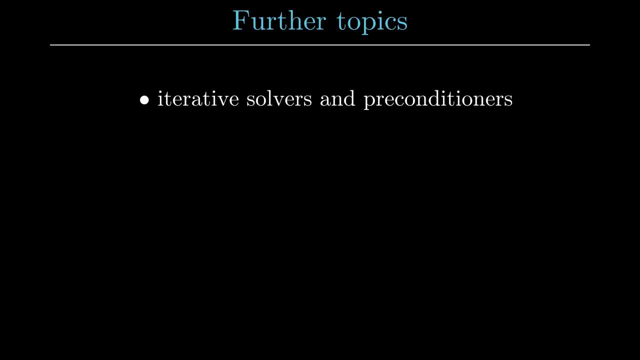 Let's look at some iterative solvers and how you can speed them up by choosing a decent preconditioner for this method. There are many iterative solvers that arise from decomposing the domain into different parts. The most prominent such method is the Multigrid method, where the PDE is being solved. 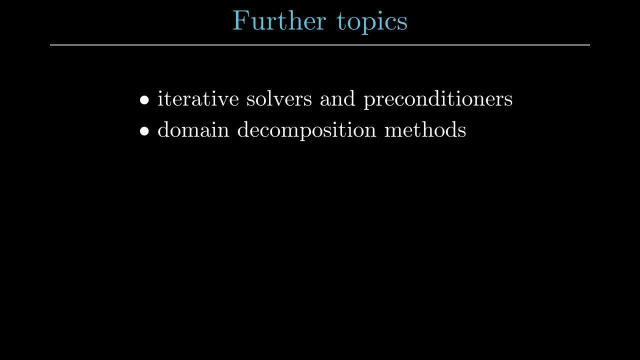 on meshes which have been refined a different number of times. Often the solution of the underlying PDE depends on the time. Thus we can say that the iterative method is the most effective method to solve linear systems. time and one might need to not only discretize the PDE in space, as we have done in this video. 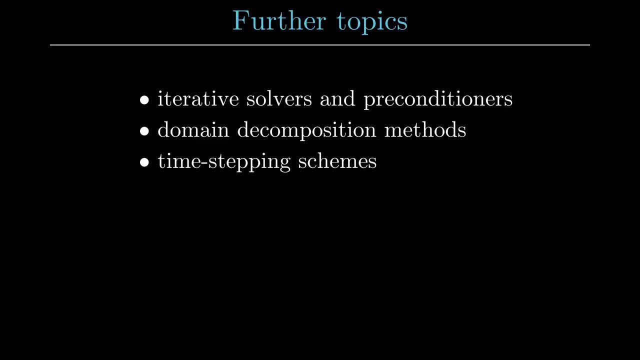 but also in time. For example, time derivatives can be approximated by the one-step data scheme. When the PDEs also contain some sort of non-linearity, then the finite element method also needs to be changed slightly. The Newton method is a good tool to solve these non-linear PDEs.